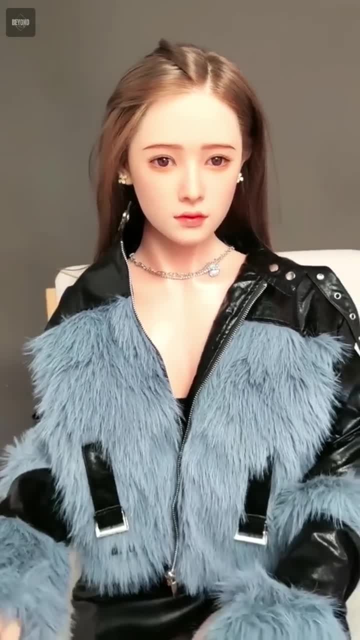 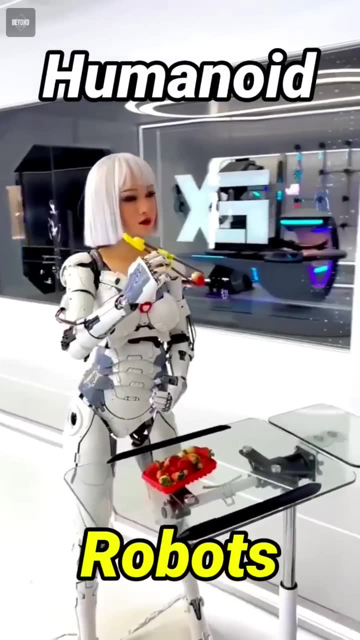 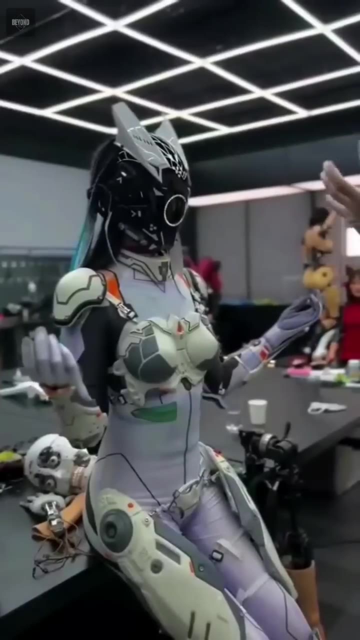 As real as it may look, this is not a real person. These are the most advanced and human-like robots in the world. These robots are called humanoid bionic robots. They are so advanced that they can exhibit human-like expressions with ease, depending on the situation These robots are. 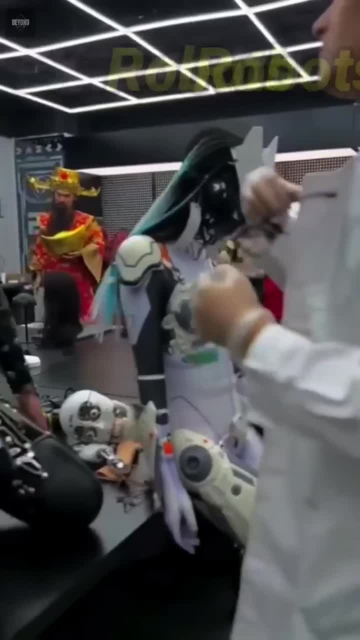 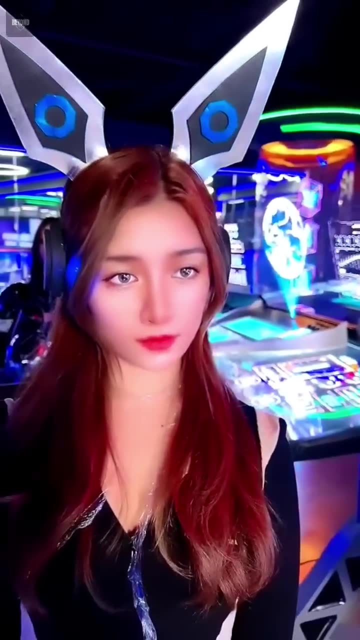 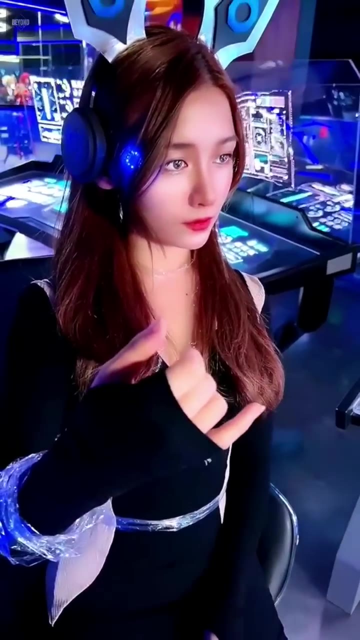 manufactured by Yex Robots, a robotic technology-based firm based in China. These robots have exactly the same face as a real person. Their faces have delicate skin, good elasticity and true touch. They are a masterpiece of silicone art, which is a combination of aesthetics and 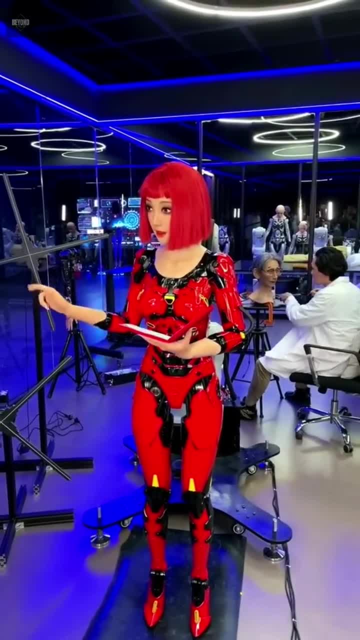 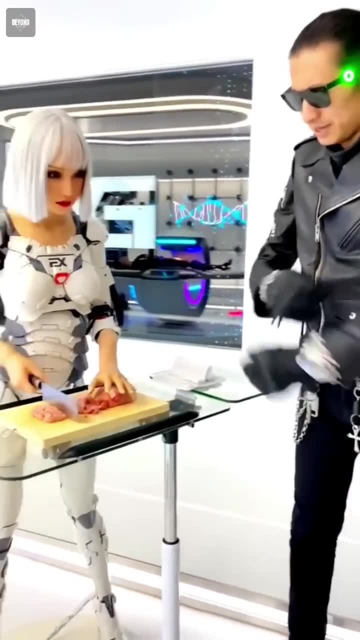 technology. Not just that, there are dozens of micromotors installed inside which allow the robot to make complex expressions showing motions and speech movement. So is this the future of robotics? 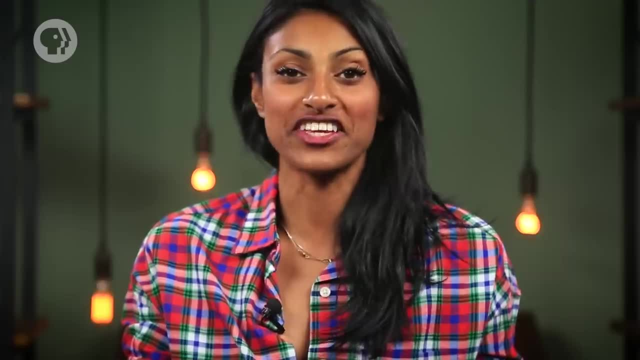 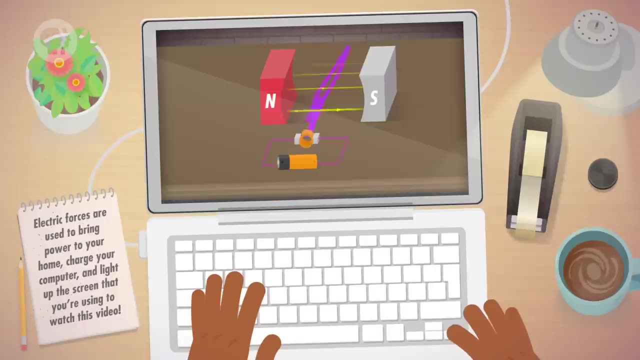 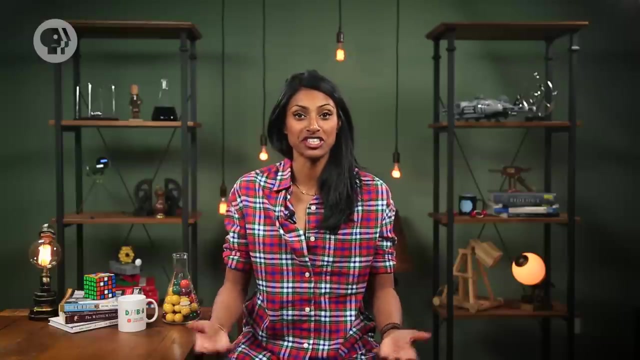 After a year of studying the laws of the universe together, a year of studying and calculating, learning about motion and fluids, thermodynamics, electricity and magnetism, light and sound, we find ourselves here: space, the final frontier. We're all voyagers on a mission to understand the universe using the power of physics. 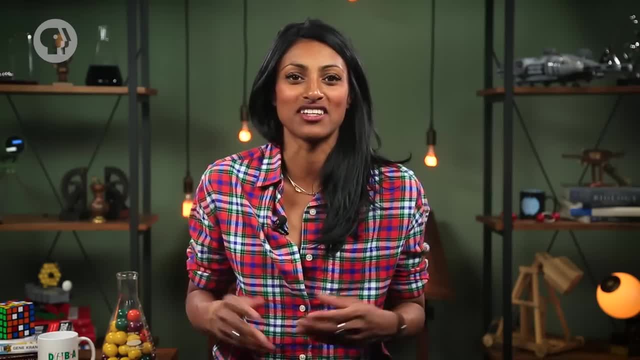 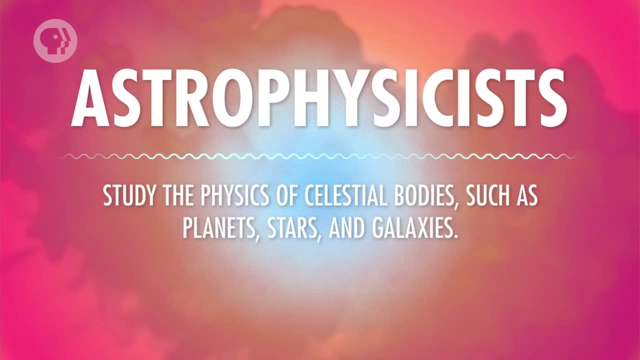 And even though we've been doing it for centuries, there's so much we have to learn about the cosmos. Some of the most exciting research in physics today is being done by astrophysicists and cosmologists. Astrophysicists study the physics of celestial bodies such as planets, stars and galaxies. 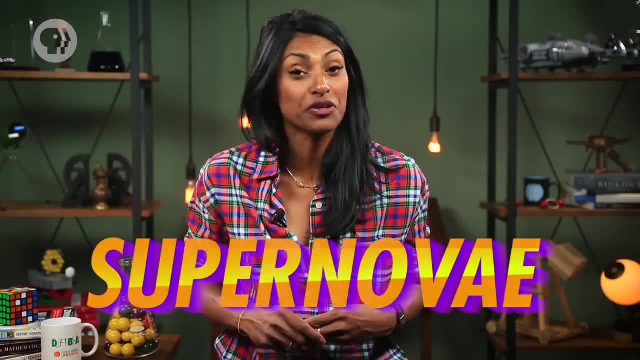 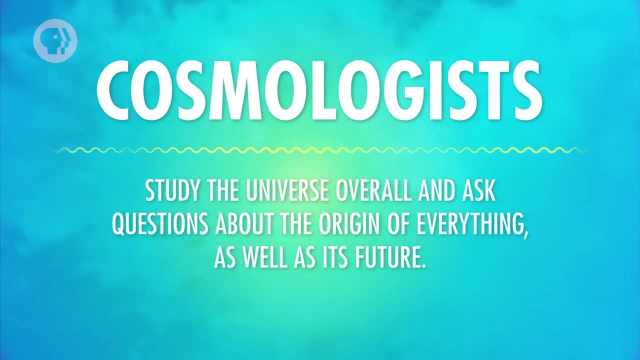 Their research takes us inside phenomena like black holes and supernovae, but we can use physics to try and understand even bigger questions about the universe. Cosmologists study the universe overall and ask questions about the origin of everything, as well as its future. 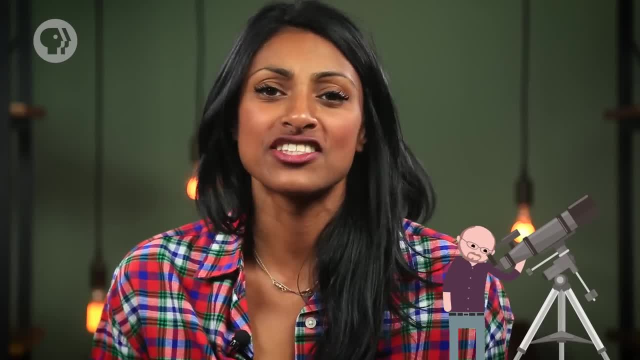 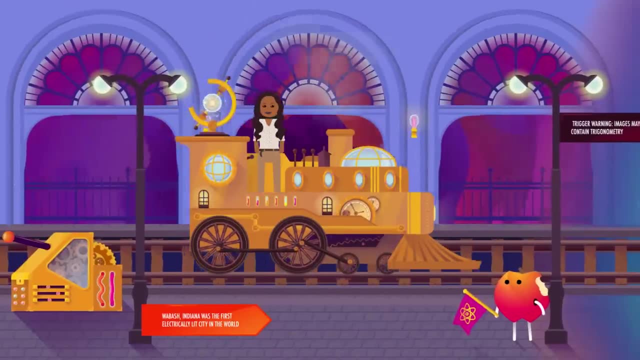 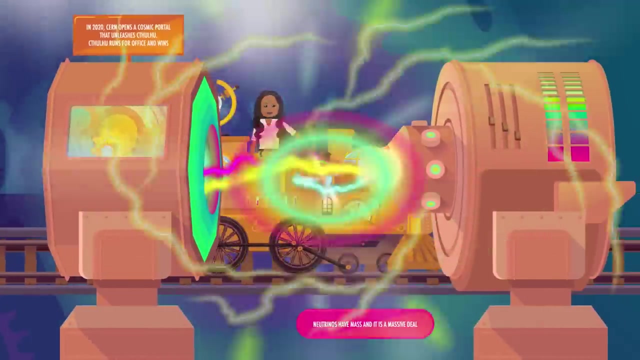 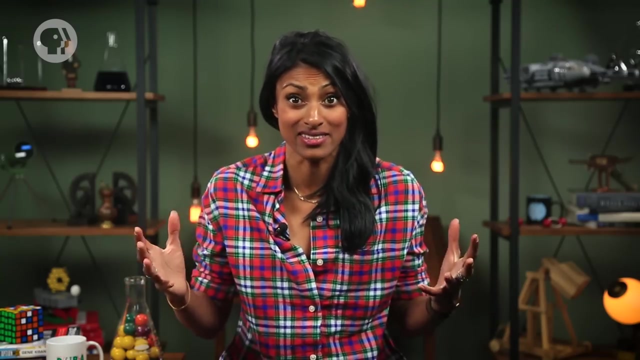 It's their job and yours to continue looking into the night sky, searching for answers using the tools we've been given, tools and knowledge that physics can provide. Before we can talk about something as big as the universe, we need to be able to describe just how big it is. 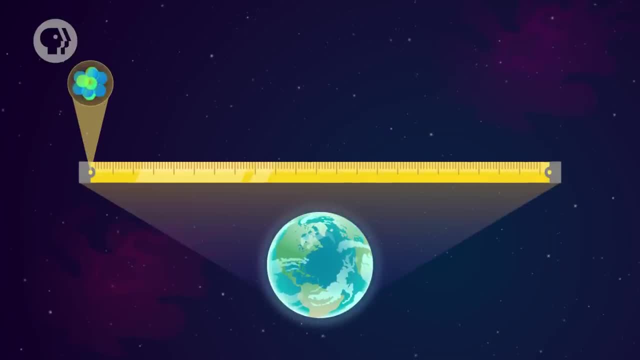 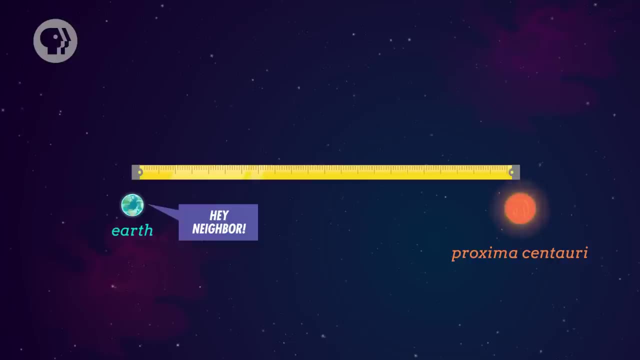 When talking about things on Earth, we typically use measurements in the range of nanometres to kilometres, But when we're in space, we need something a whole lot bigger. For instance, I could say that the nearest star to the Earth, which is the nearest star to the Earth?